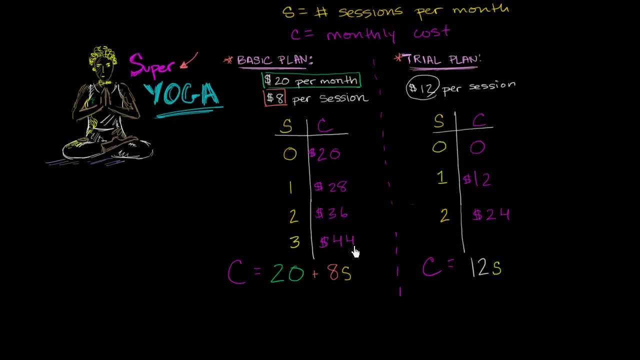 Now, let's do the same thing under the trial plan. How much is it going to cost us to attend three sessions? Well, this is more straightforward, or slightly more straightforward. Our total cost is going to be equal to 12 times the number of sessions. 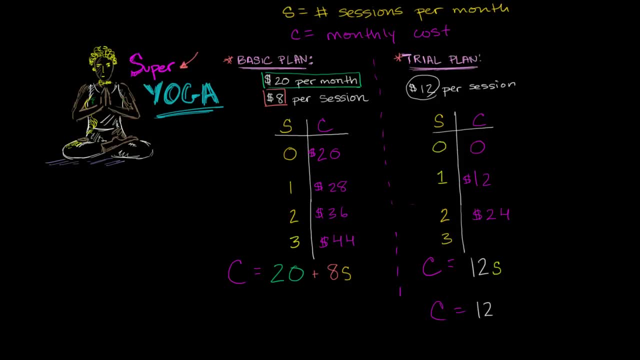 The number of sessions in this circumstance are three sessions, So it's going to be 12 times 3.. So our total cost is going to be equal to $36.. So let me write that down. So it's going to be equal to $36.. 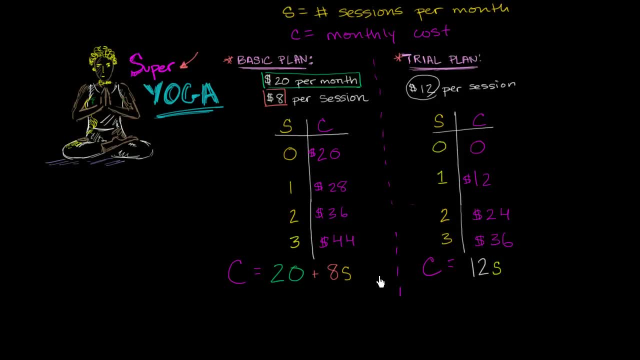 But we could also answer more interesting questions with these equations. For example, how many sessions can I attend in a month for, oh, I don't know. let's throw out something for $54?. Let's say that's just my budget. 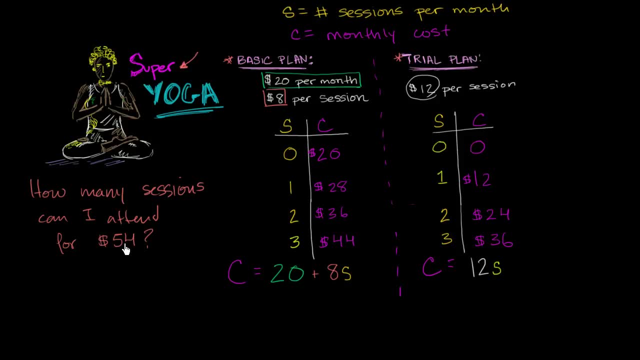 When I look at my salary and how much money I have budgeted to health and fitness, this is what I can afford, And so, based on that, I want to ask: how many sessions can I attend in each of these situations? So first let's think about it for the trial plan. 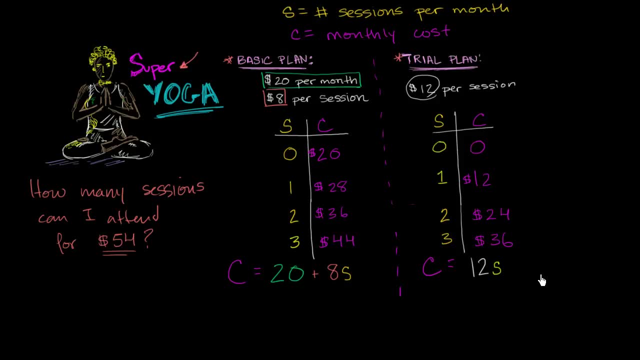 How many sessions can I attend for $54?? And let's just assume that this is some type of a special yoga studio where you can even attend half a session. So if you attend half a session, they'll charge you $6.. If you attend a fourth of a session, they'll charge you $3.. 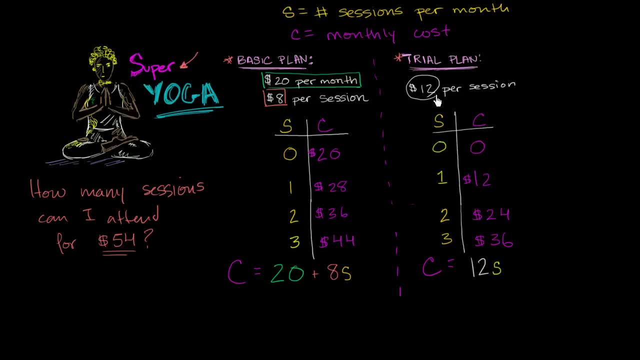 So they'll actually keep track of exactly what fraction of a session you're attending, So you don't have to just attend a whole number of sessions. You could attend two and a half, and they'll bill you accordingly. So, with that said, how many sessions under the trial plan? 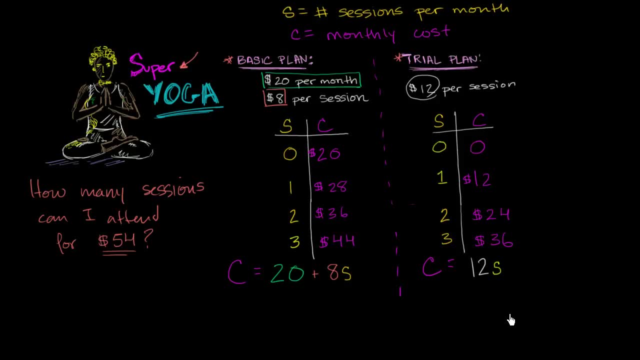 can I attend for $54?? Well, let's think about this a little bit. So my cost now is going to be $54.. $54 is C, It's my monthly cost. So $54 is going to be equal to $12 per session. 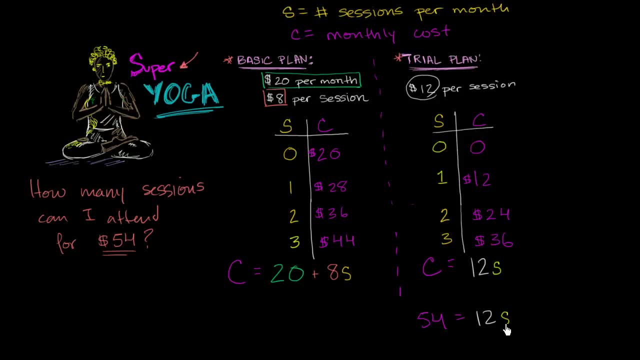 times the number of sessions. So now I've set up this equation In order to answer this question. I just need to figure out what's the number of sessions that satisfy it. Now this S is an unknown variable. What number of sessions times 12 is equal to 54?. 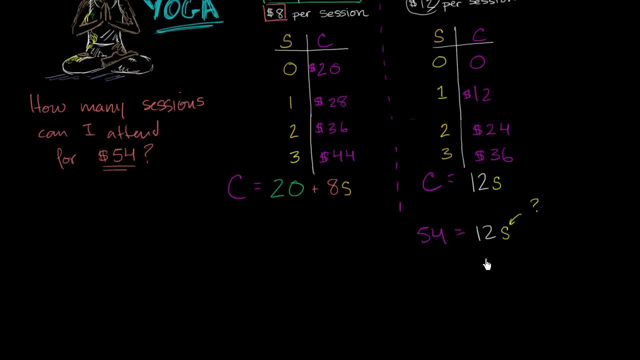 Well, you might say: well, if I could just get an S, just an S on the right-hand side here, then I'll have an answer. S will be equal to some value. And if I want just an S on the right-hand side, 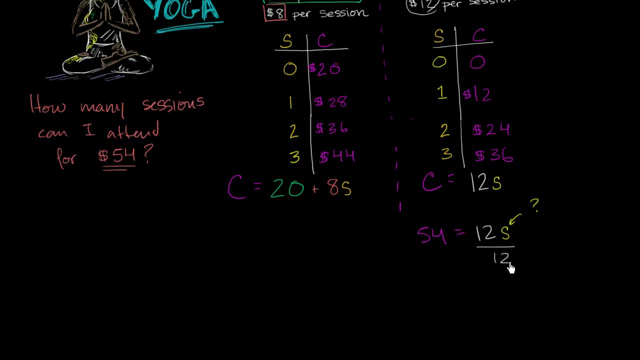 I'd ideally just like to divide this by 12.. 12S divided by 12 is just going to give me an S. It's just going to give me the number of sessions. But if I have an equal sign, I can't just willy-nilly. 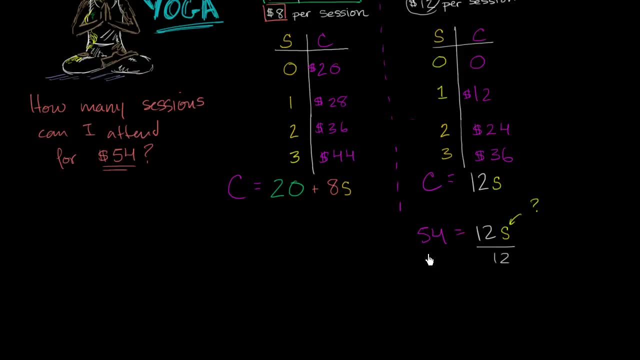 divide one side by 12 without doing the exact same thing to the other side. If that is equal to that, in order for them to both still be equal, I have to do the same thing to both. So on the right-hand side, I am left with just an S. 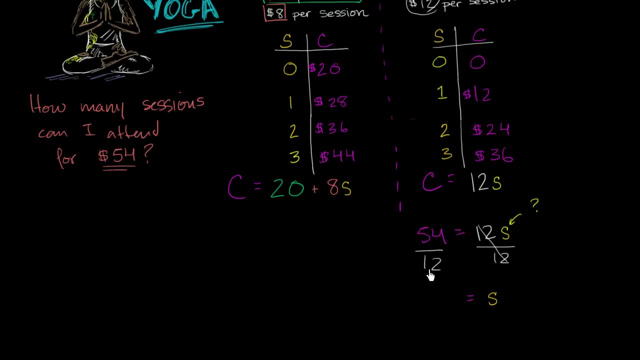 And on the left-hand side I have 54 divided by 12.. Let me think about that. 12 goes into 54.. I'll just work it out: 12 goes into 54 four times. 4 times 12 is 48.. 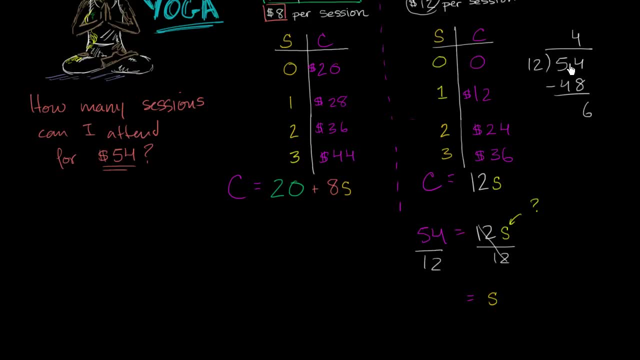 You're left with a remainder of 6.. So you could say: 12 goes into 54. Or you could say 54.. 4 over 12 is equal to 4 and 6 twelfths, or 4 and 1 half. 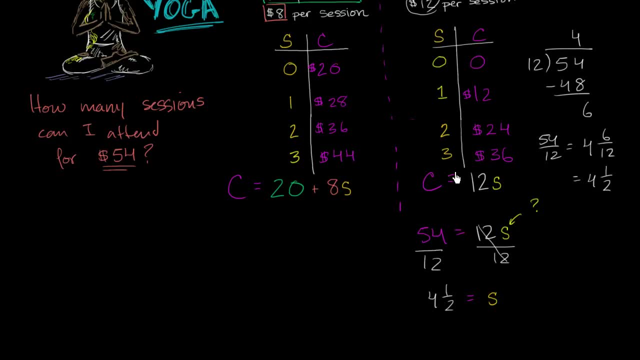 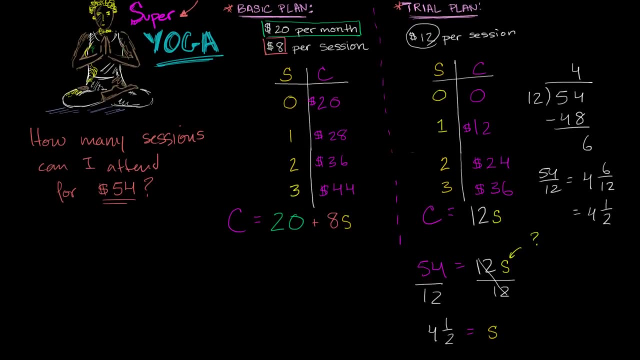 So the number of sessions that I could attend are 4 and 1 half. If I have $54 to spend, I could attend 4 and 1 half sessions under the trial plan. If this was a yoga studio, that said, oh you. 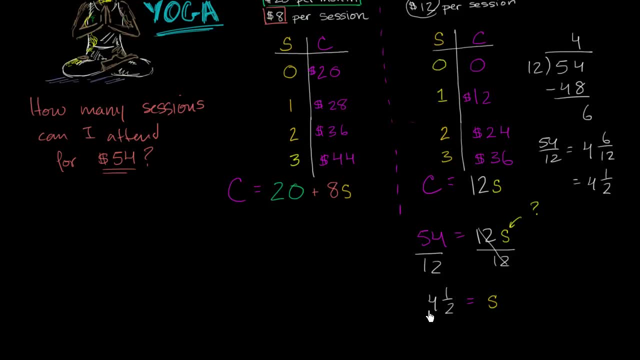 can't attend half sessions. then you could say: well, at most I could attend four sessions, Because five sessions would get me above my budget. But I said that you can attend fractional sessions, So we're going to say 4 and 1 half. 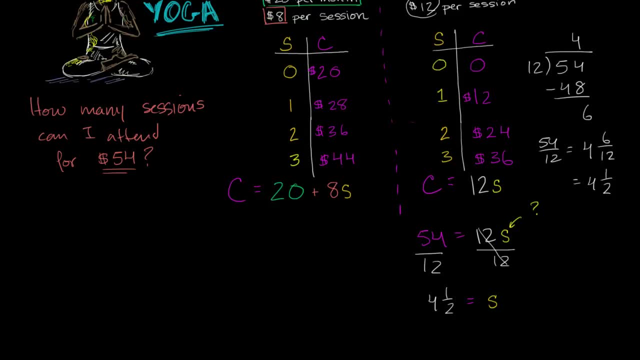 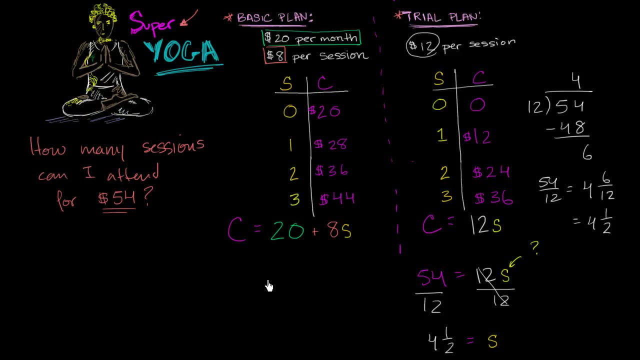 Now let's do the same, Let's answer the same question for the basic plan. Under the basic plan, how many sessions can I attend for $54?? Well, once again, this is going to be our cost, our total cost for that month. 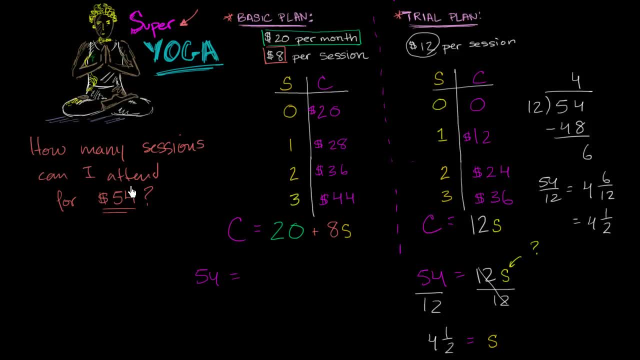 So we say $54 is equal to 20 plus 8 times the number of sessions. And once again, I'd like to just have sessions, maybe on the right-hand side of this equation, So I could say: oh, sessions are going to be equal to something. 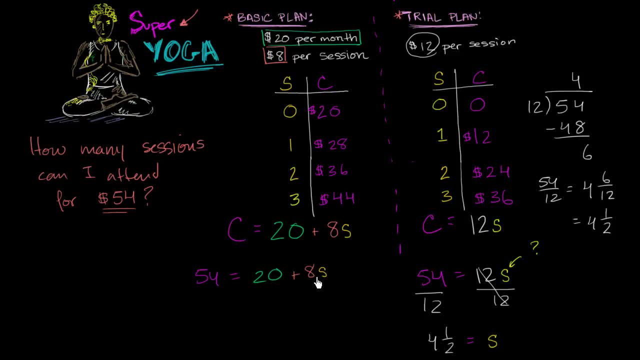 This is the number of sessions that I can attend, But I have this 20 here and this 8 here, And so I have to think about how I can get rid of them. So the first thing I think about is how can I get rid of this 20 from the right-hand side? 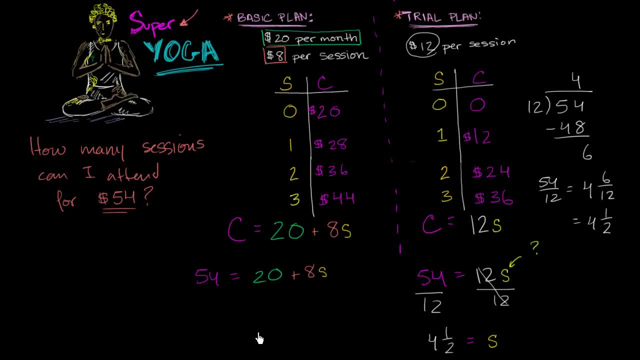 of this equation. What am I going to have to do to the entire equation? Well, the simplest thing is: I could subtract 20 from the right-hand side, But if I subtract 20 from the right-hand side, I also have to subtract 20 from the left-hand side. 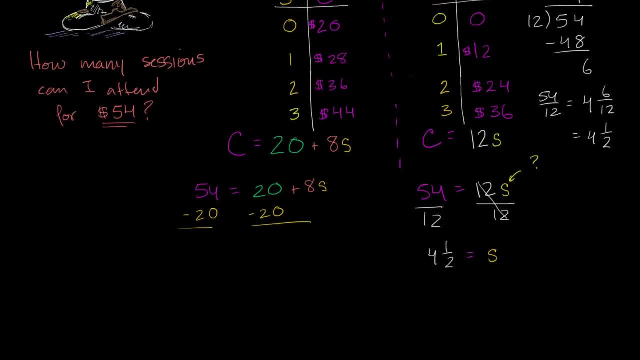 in order to maintain the equality, And so I'm left with, on the left-hand side, 54 minus 20 gets me 34. And that's going to be equal to well. the whole point of subtracting 20 is so that these negate each other. 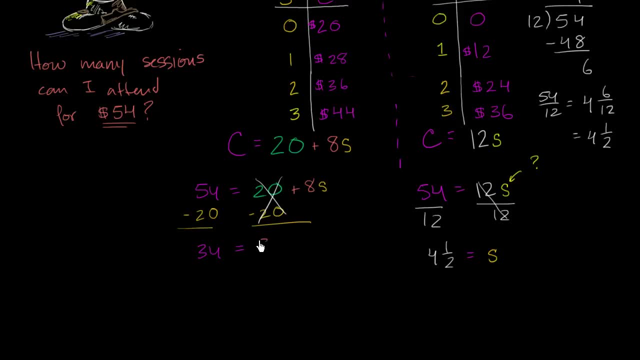 And then I have just an 8s. It's just 8s. So 8 times the number of sessions has to be equal to 34.. In order for 8 times the number of sessions plus 20 to be equal to 54.. 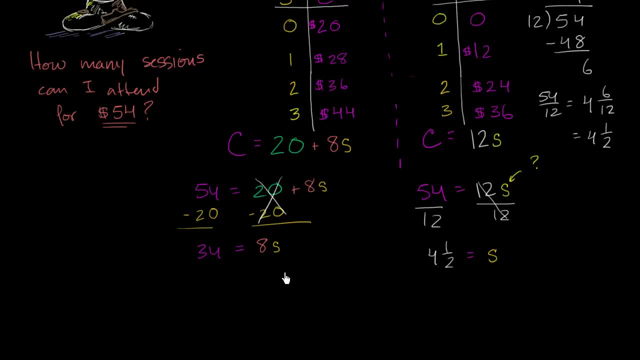 And you could add 20 to both sides of this equation to get our original. So we're almost done. We just want to isolate the s right here And you can imagine the easiest way would be to divide the right-hand side by 8.. 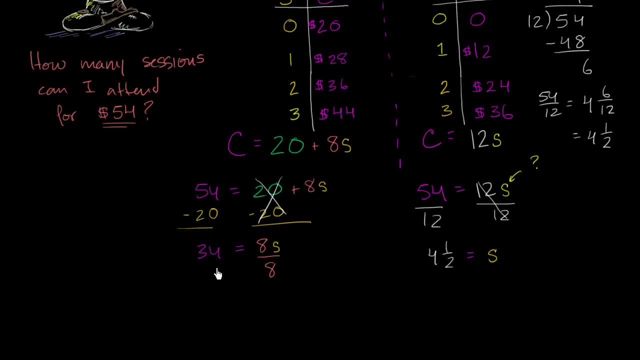 But if we're dividing the right-hand side by 8, we have to do the same to the left, And so what do we get for the number of sessions that we would have to attend? Well, these cancel out, And so you get. 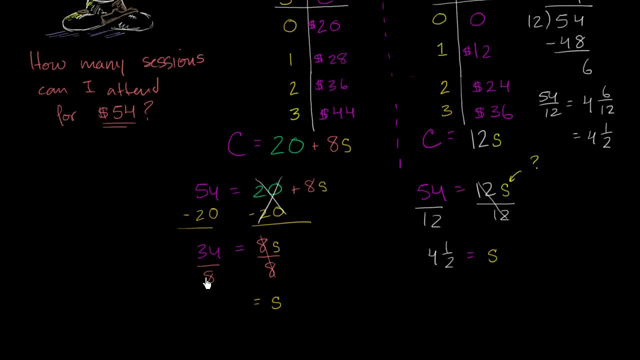 You get the number of sessions is equal to 34 divided by 8.. 34 divided by 8 is equal to: let's see: 8 goes into 34 four times, with the remainder 2.. So 4 and 2 eighths, or it's 4 and 1 fourth.